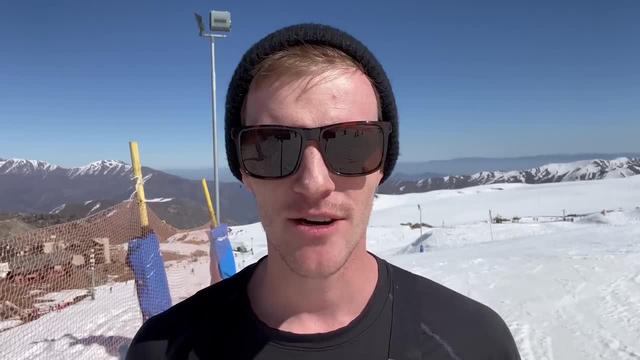 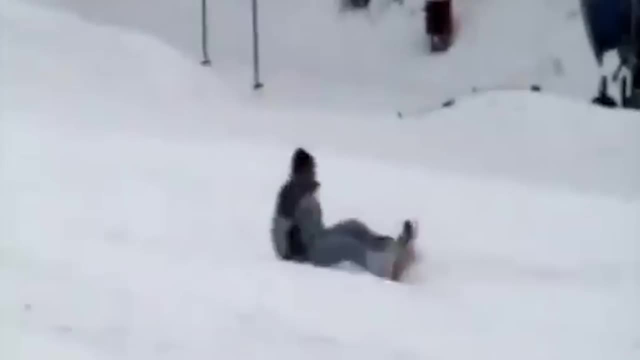 turns and all this stuff, but they're still a beginner. But I'm going to go ahead and say a beginner snowboarder is somebody who doesn't know the basics. They don't know how to push with one foot in, They don't really know how to position themselves on the mountain to even stand up on. 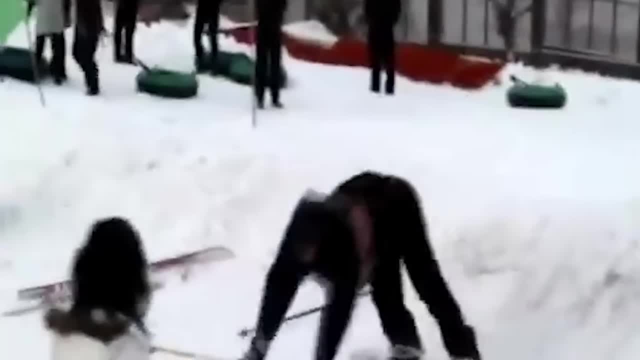 their snowboard. If you've ever watched beginners, this is really hard for them. They struggle with putting their bindings on, They don't know how to link turns or they're just learning. So I think that you graduate from being a beginner when you can consistently. 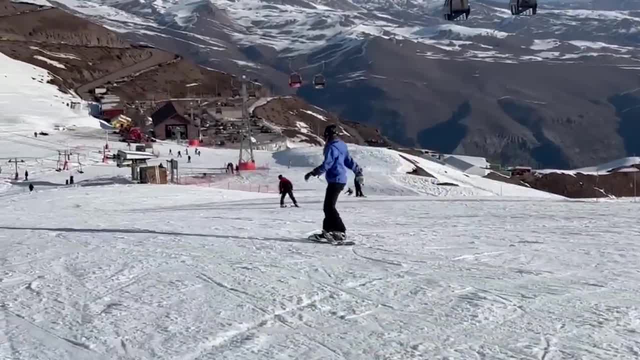 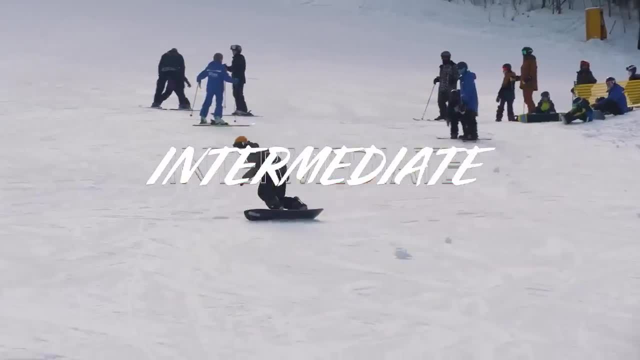 link turns heel side to toe side. If you're just doing falling leaf, you're still a beginner. As soon as you transition to I can ride down green circles and maybe even some mellow blue squares linking heel side to toe side turns. then you're intermediate, because you're so much better. 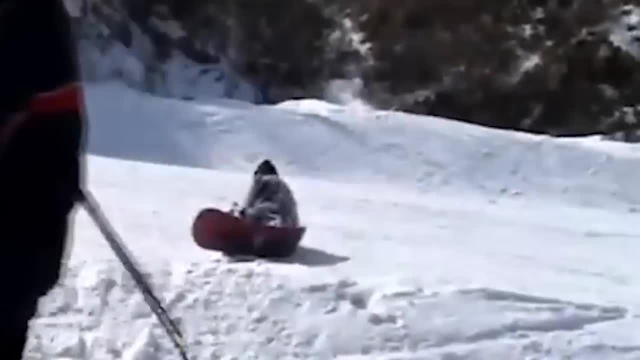 than somebody who doesn't know how to stand up on their snowboard, who doesn't know how to link turns together. Okay So, beginner snowboarder, still learning the basics: how to get on and off the lift, how to ride with one foot. 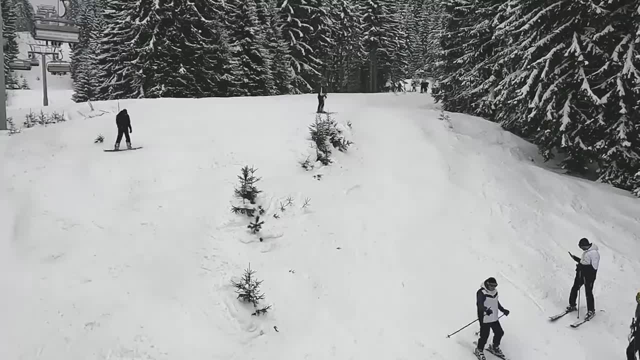 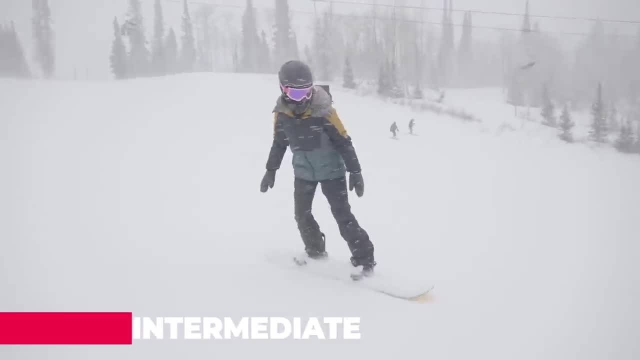 how to link those turns, do falling leaf, all that kind of stuff. Once you have those basics dialed, the basic fundamental building blocks of snowboarding, you're now intermediate And getting from intermediate to advanced is really about perfecting those building block. 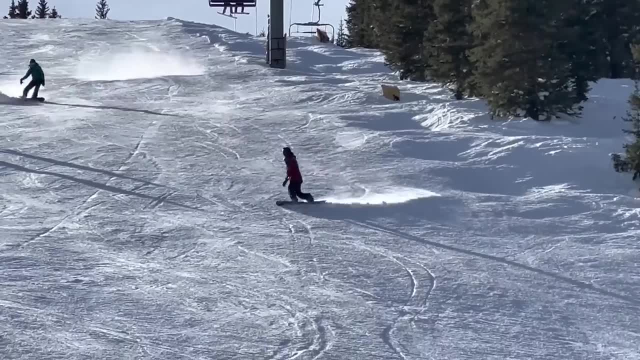 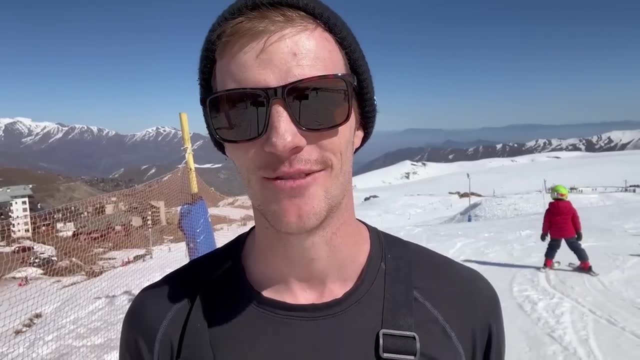 skills It's about. can I link heel side to toe? side turns down blue squares and maybe even groomed black diamonds. Can I get down the mountain every single time without eating and hurting myself right? Can I get on and off every lift with one foot? Can I get on and off every lift? 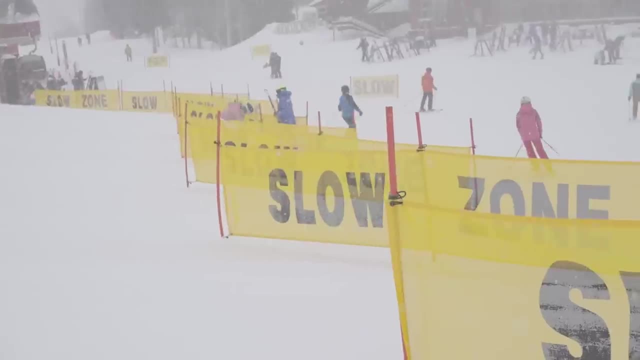 with one foot. Can I get on and off every lift with one foot? Can I get on and off every lift with confidence? Do I still fall on the left sometimes, Cause I know some people have been sowing for years and they still fall, getting on flip. I would call that person intermediate. 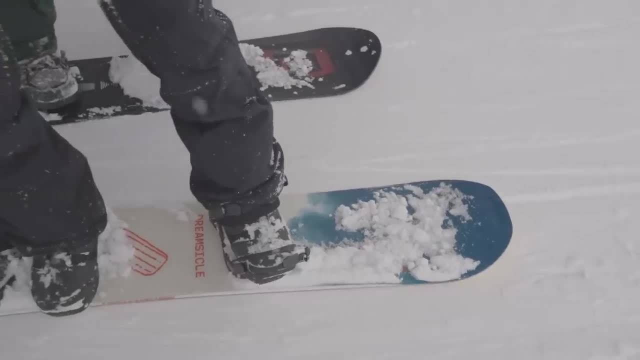 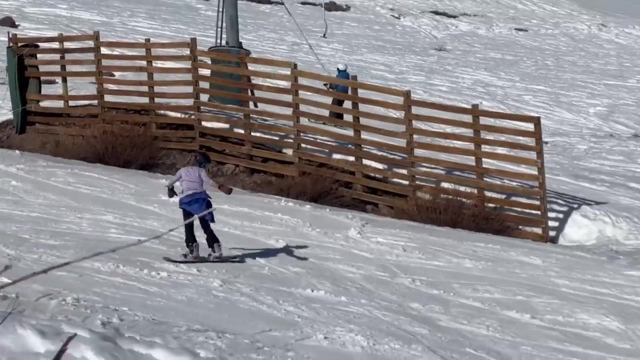 They're never going to be advanced if you're falling every time you go down the mountain. So mastering those skills on different types of terrain, in different conditions, different weather, different resorts, and being able to consistently do it every time, that's what's going. 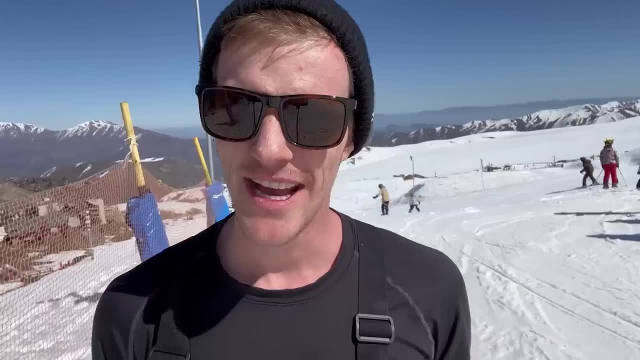 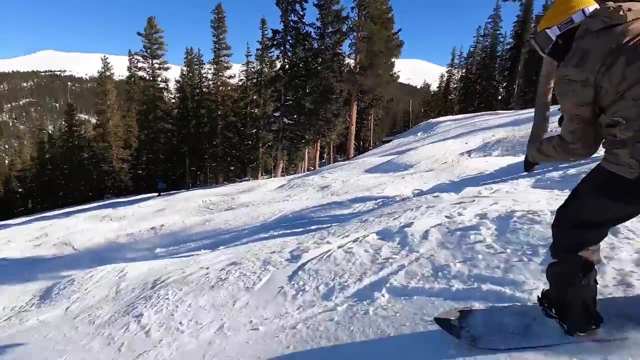 to take you from intermediate to advanced. Now I really don't think you can call yourself advanced in snowboarding until you can carve across the whole mountain down black diamonds. So you learn to ride bumps and trees and variable terrain till you can ride in the pow right. these are all still. 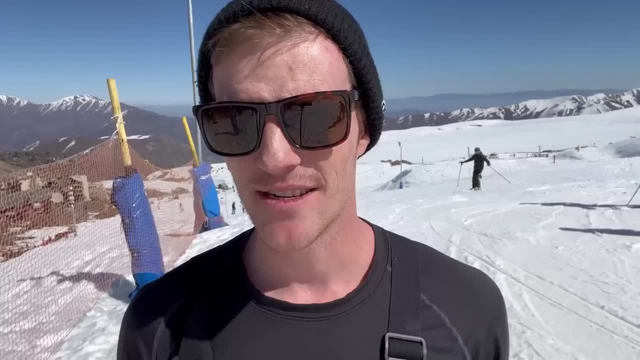 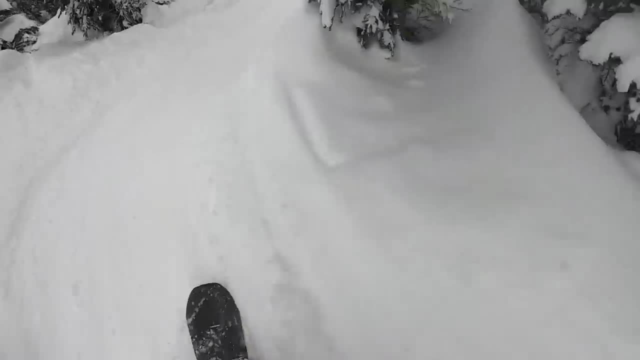 just basic building blocks of snowboarding, but they're a lot more advanced than a beginner or an intermediate person would be able to ride. so this means you can ride the whole entire mountain consistently, with confidence. you can link turns down any kind of slope. you can ride those moguls. 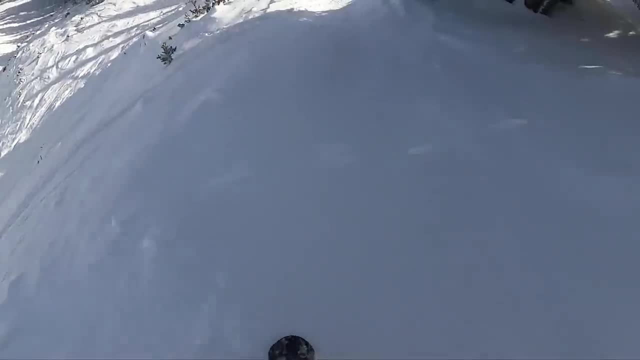 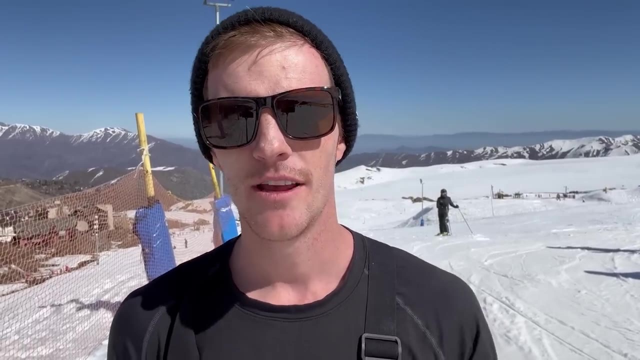 those bumps, those trees, that pow. a lot of people get pretty good snowboarding. then a pow day comes and they're lost, right. so this is advanced, it's really mastering these skills and there's a whole spectrum- right, you might be beginner level, advanced- where you can ride trees, moguls, but 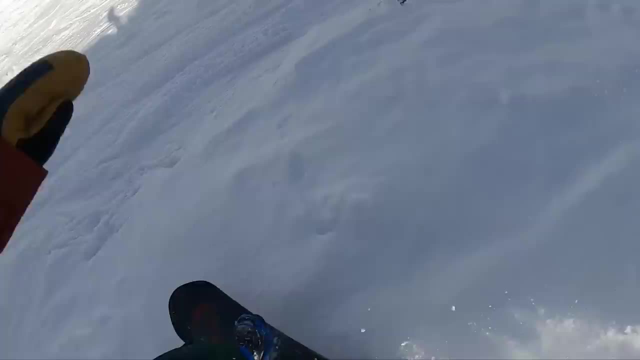 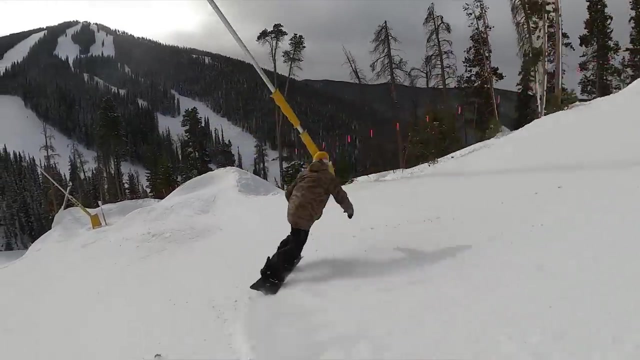 you get scared every once in a while, you really have to slow yourself down, and then there's riding that with confidence. that's a whole new level. and then we have the expert snowboarder now on the internet. there's a distinction between an expert snowboarder and somebody who's actually an expert. 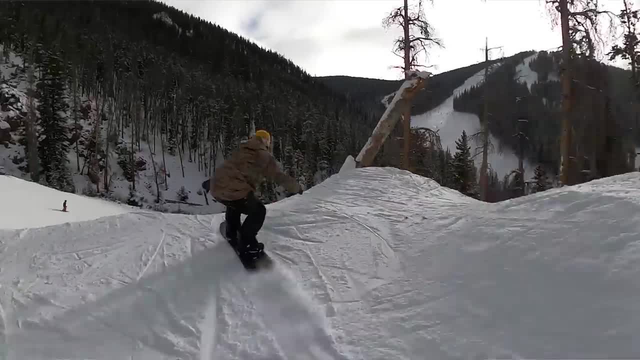 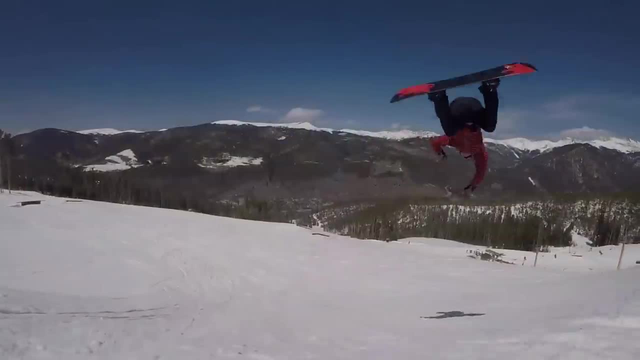 at snowboarding. so i think a lot of people probably on watching this video think that they're an expert and i would agree in some sense. and in another sense i would disagree, because are you an expert if you can't do a 900 off a park jump? 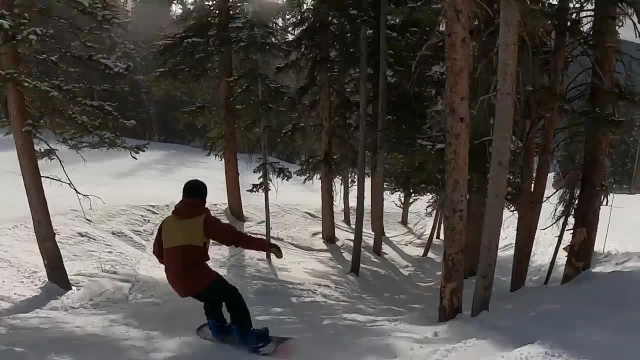 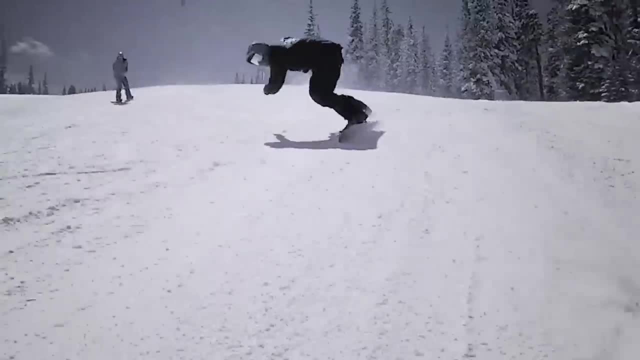 and if you are, if you're an expert just because you can ride pow and bumps and trees and all those things, how do you distinguish between you and somebody who can do a 900 or double cork right? this curve just keeps going and going and the learning curve at the beginning is like kind of 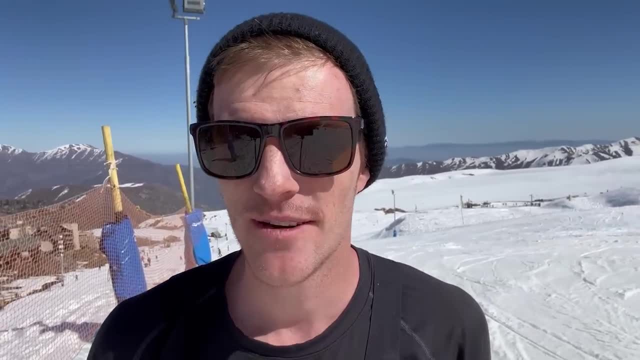 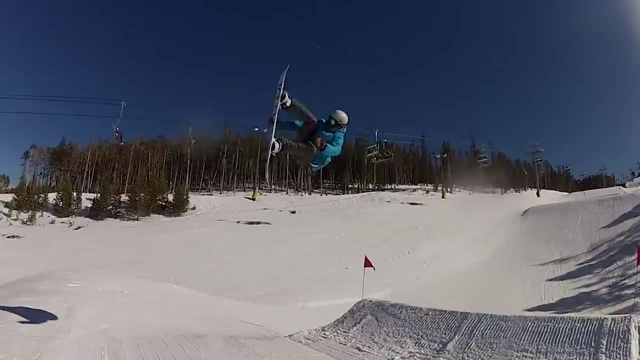 flat. you're getting better and better, but at the end the top 0.5 percent of snowboarders are so much better at snowboarding than the top two percent or the top five percent. so what do we call those? i guess we call them pros in some instances, but not all of these people are actually professional. 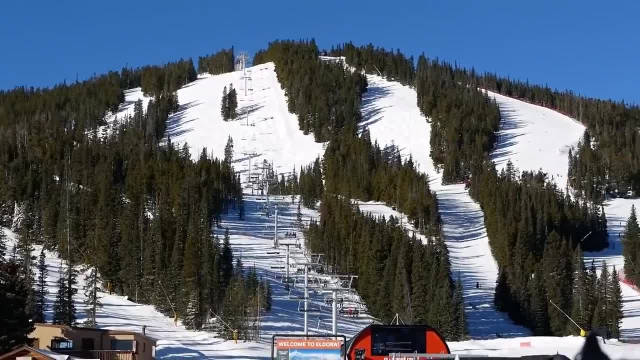 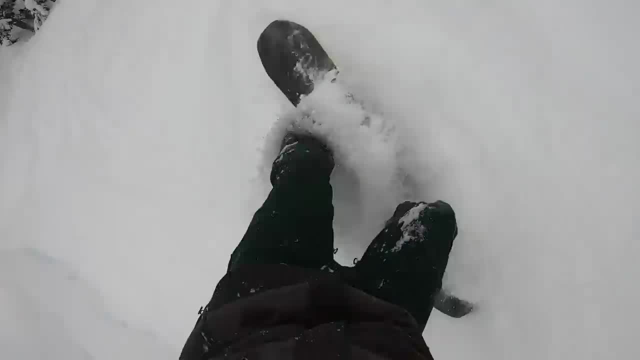 snowboarders. so to be an expert snowboarder, i'm going to go ahead and say: you have to do the first thing you're going to do in order to be able to charge the whole mountain. that means you're riding mogul fields, but you're also popping ears in between them. right, you're riding trees and 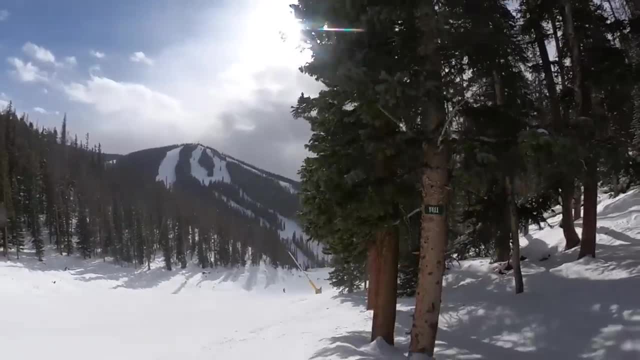 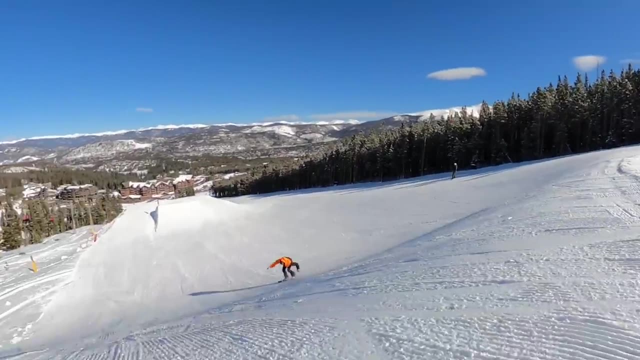 you're slashing pow in the middle of it. you're throwing 360s off of cut-ups, your air and over stuff. you're all in fences. right, you have some freestyle tricks in your bag. it doesn't mean you can roll into the park and throw down a 720, because usually you have to ride park every. 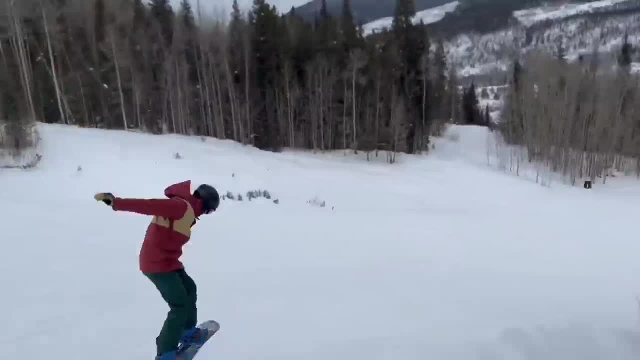 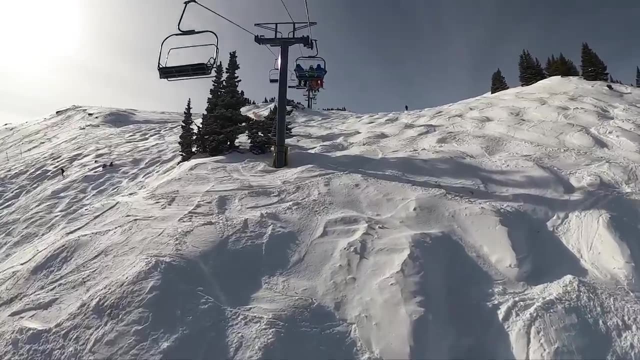 single day and really live the whole lifestyle. so i think you can be an expert snowboarder if you can charge the whole mountain and do freestyle tricks around the mountain and you can black diamonds. that would be an expert in my book because it's so much further than just somebody. 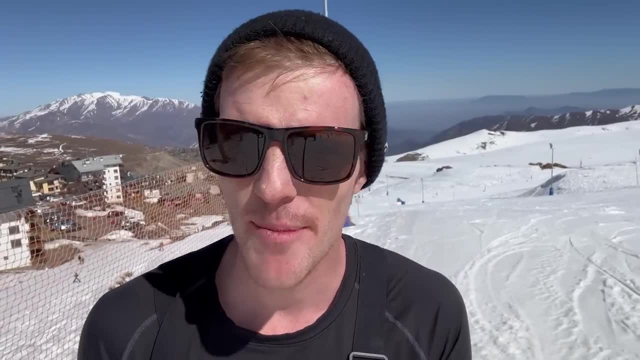 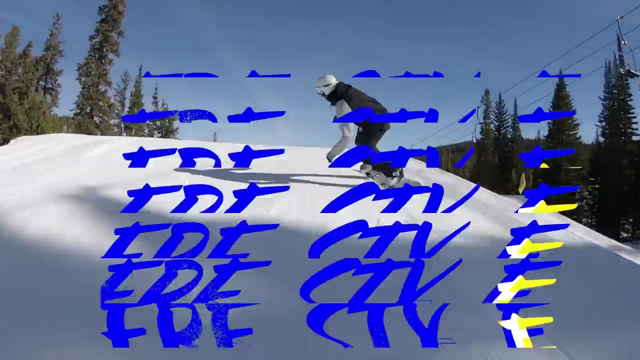 who's advanced and can ride all the terrain, but can't ride switch, can't pop an ollie over a mogul. as soon as things get bumpy, they peace out. we've got the expert rider, so i'm going to go ahead and put freestyle in a category of its own. it's almost as if you have to work through the ranks of all. 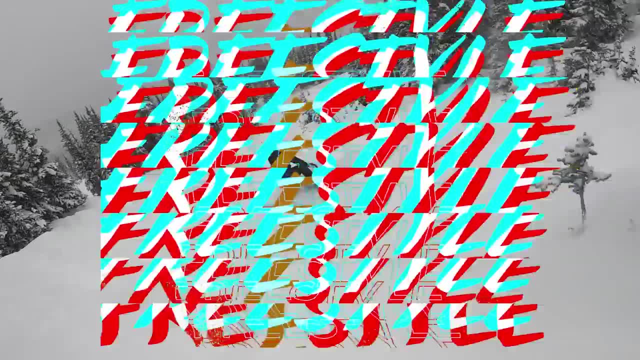 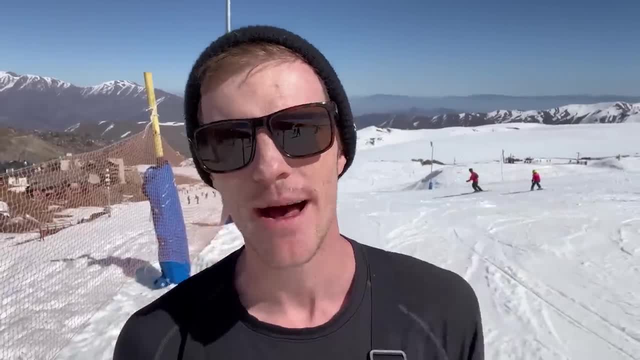 kinds of snowboarding, from beginner to expert, and then we add our beginner level freestyle. this is learning how to hit jumps, rails, boxes, because i know you guys know some treaders, some of you out there are absolute shredders. but you wouldn't step foot in the park, you wouldn't grind a rail. 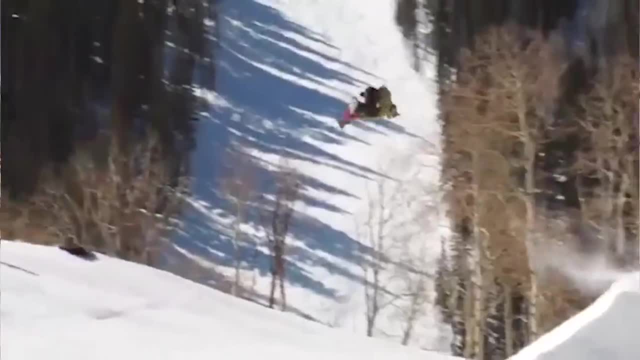 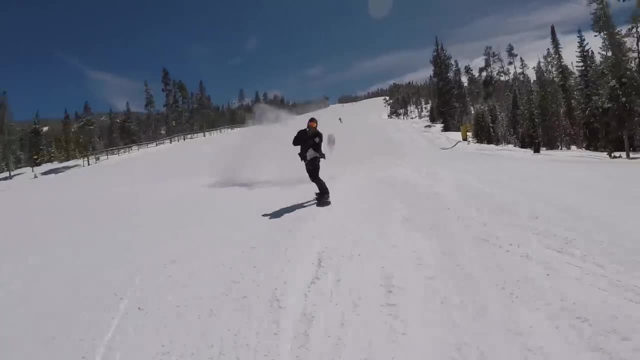 you don't know how to board slide and you wouldn't do a 900 over a 60 foot jump. that doesn't mean you're not an expert snowboarder, but it means you're beginner level freestyle. you're the same person who can't get on the lift yet, but in a completely different category, somebody who, when 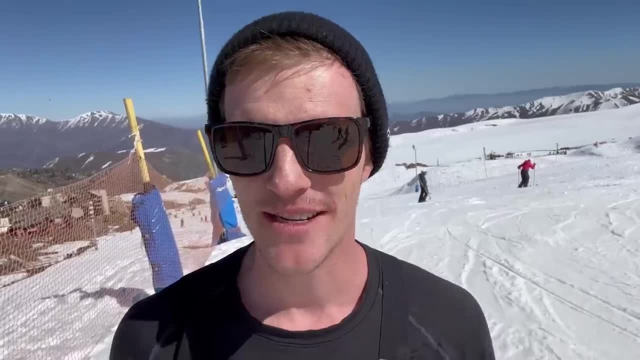 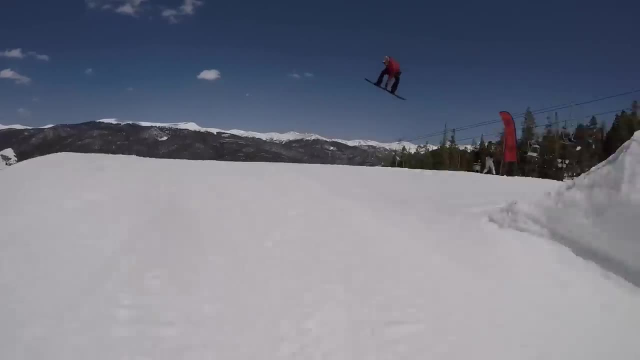 we bring you into the park. we're starting at ground zero with those fundamentals. so i think that's the really important thing about this video is we have to distinguish between snowboarding and freestyle snowboarding. they're two completely different things, and freestyle spectrum gets just harder and harder and harder. you know, the guys at the very top are 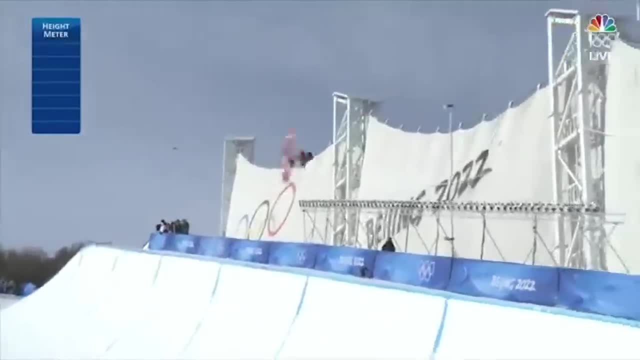 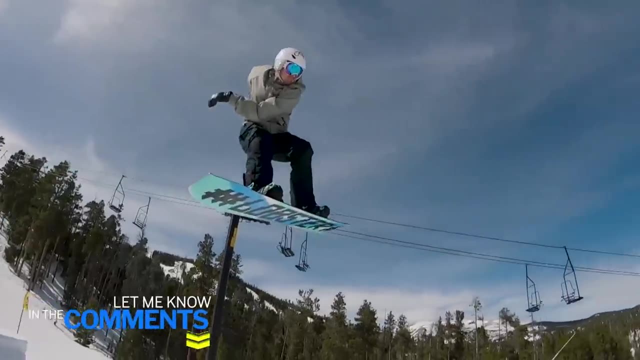 risking their lives every triple cork in the half pipe they do. that is so much further ahead than the advanced or expert level snowboarder you're going to find on your average mount. so throw in the comments. are you in just the regular snowboard category or the freestyle snowboard category? 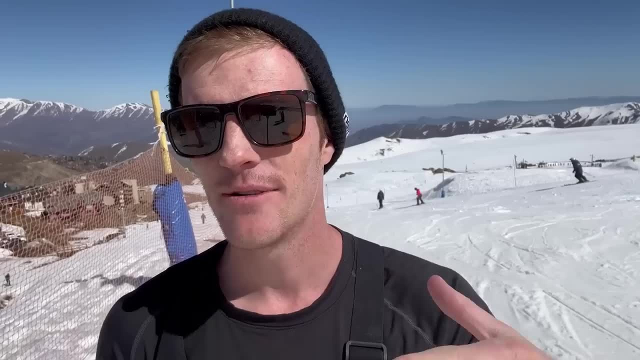 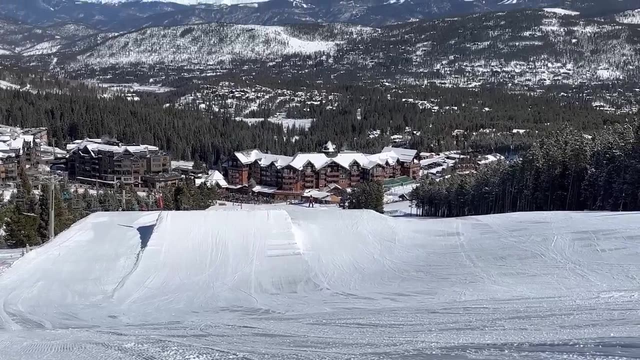 remember the freestyle beginner- or intermediate i would say- is more advanced than an expert snowboarder. so you could be intermediate freestyle snowboarder that's going to be above expert level snowboarder, which is going to be the most advanced snowboarder you're going to find on your average. 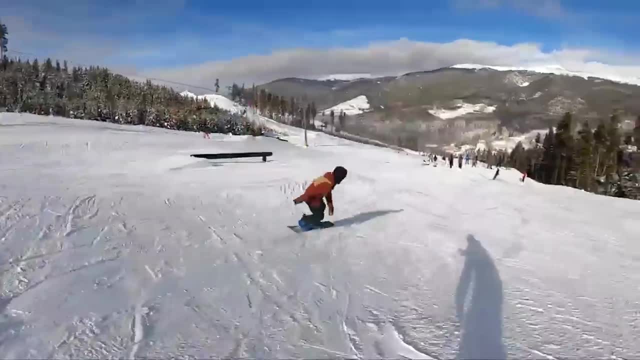 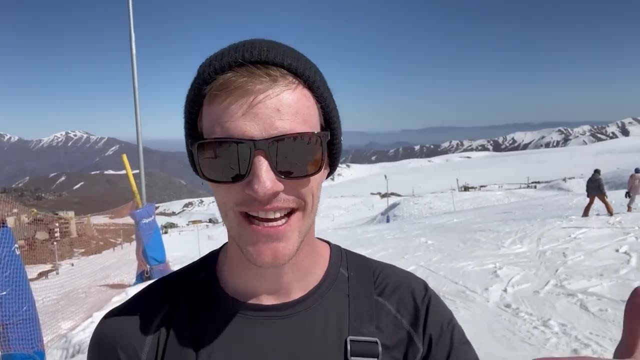 category are you in? snowboarding or freestyle snowboarding? on what level are you? i put together free quiz so that you can figure this all out without the guesswork. go ahead and just click the link in the description, take the quiz and then tell me what you got in the comments and. 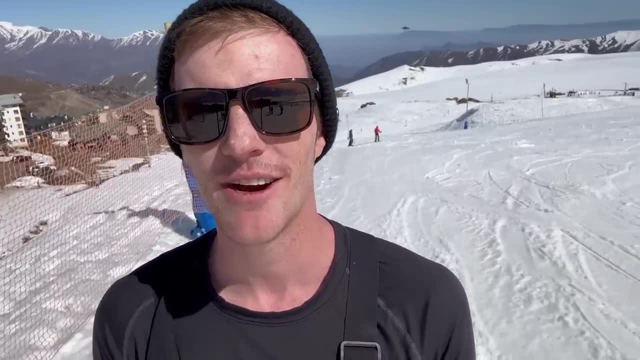 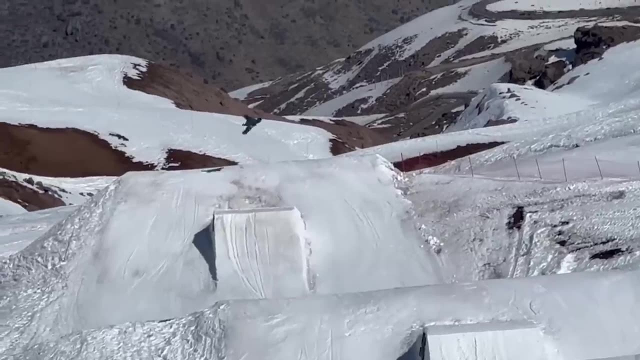 go ahead. if you have any arguments you disagree with whatever i said, i would love to hear it. i'm open to conversation on all this. that's all for today. we're in beautiful chile in august, shredding right now. what a life we live. peace out shredder. you.